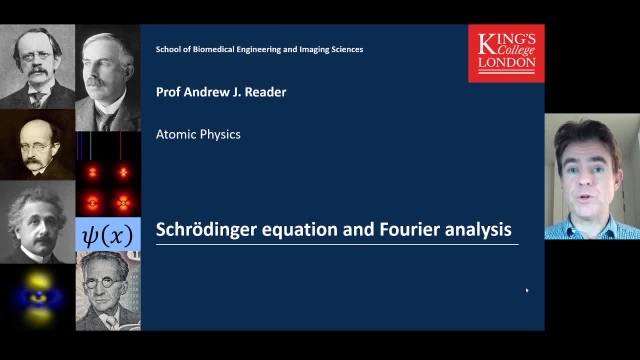 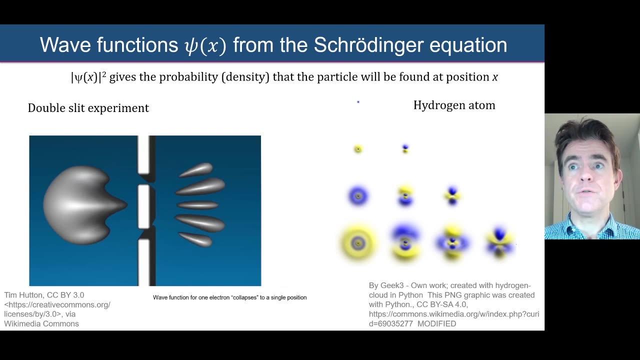 In this video I want to talk a bit more about the Schrodinger equation, specifically really solutions to it that are wave functions, and then go into Fourier analysis to help us understand those wave functions. So here then are example wave functions found from the Schrodinger equation for two particular cases. 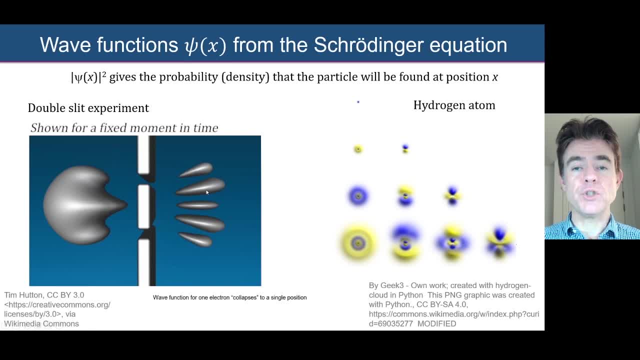 On the left-hand side, we're seeing a simulation of the double slit experiment, where we have an electron approaching a double slit and it's a wave function resulting in this interference pattern that we can detect on a screen And, of course, when the wave function is detected, it collapses to a single position that is detected. 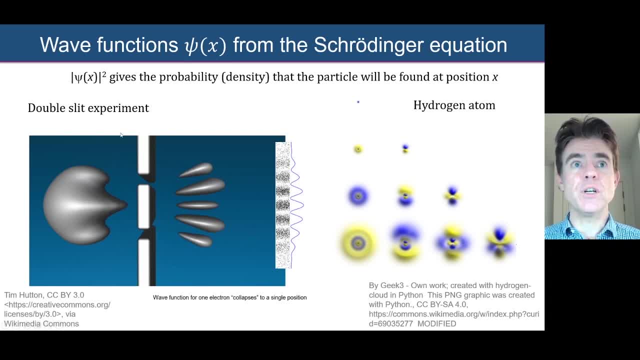 And during the experiment itself, we regard the wave function as allowing us to find the probability of finding the particle anywhere, And so it's when it arrives here that we then sample and get the probability of measuring that electron at a particular location on this detection screen. 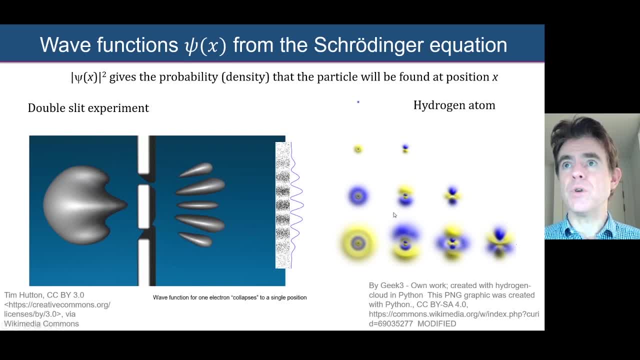 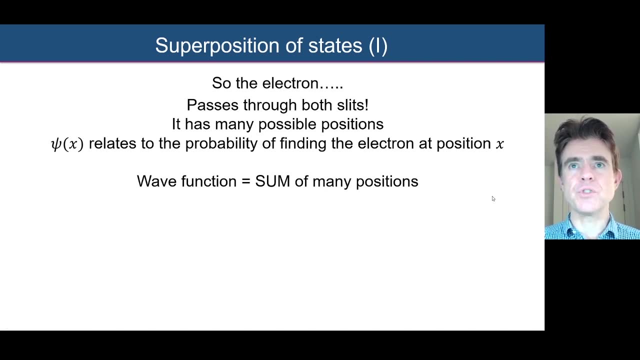 And on the right-hand side we have example solutions to finding electron orbitals for the hydrogen atom, and so I refer you to an earlier video to look more at those in detail. So, looking at that double slit experiment with the wave function passing through the two slits and being detected, 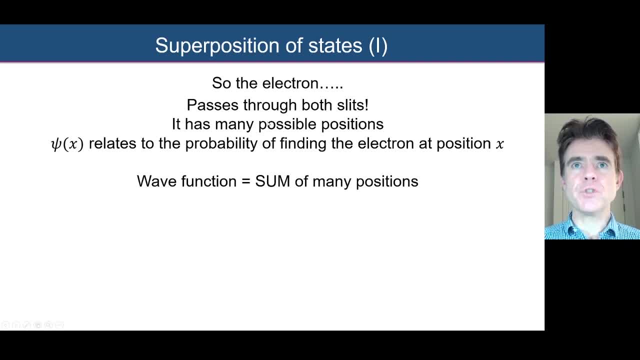 in a single position on the screen, we have to conclude that that electron, as a wave function, is passing through both slits, as we've seen before and as we saw in the previous slide, the animation of that wave function rebounding and also partly passing through and interfering with itself. 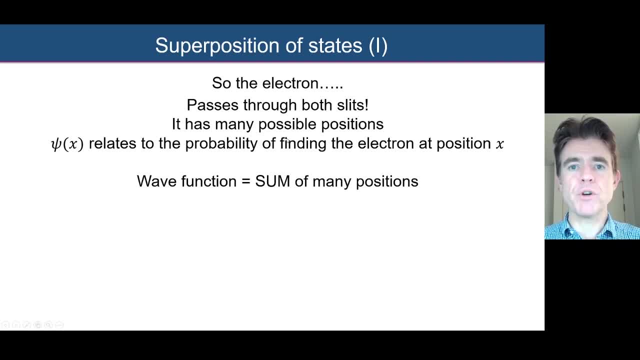 So therefore, it has many possible positions where, if we tried to measure where the electron was at any given moment, we could end up with it being found anywhere according to a wave function. So that's why the wave function relates to a probability amplitude given by that wave function form that we've seen. 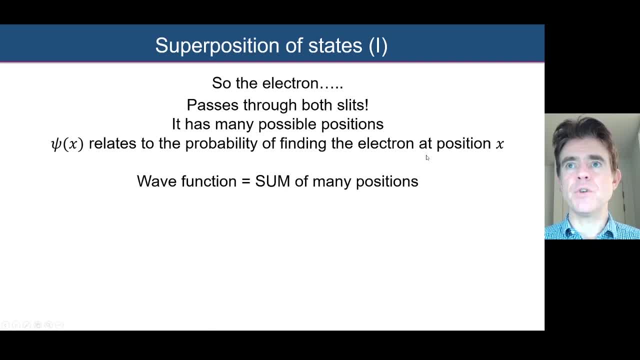 And so that's why the wave function relates to the probability of finding the electron at that position, at a position x, And so we say that the wave function is a superposition or a summation of many possible position states. So in mathematics that means the wave function is equal to a summation, a superposition of position states. 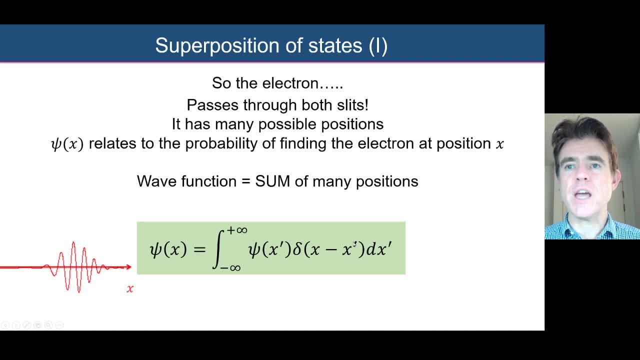 Here is one position state: delta x At position x prime. that's like a spike function. Here we have a general wave packet which is composed of many of those delta spike functions, And here we're just looking at one of them. 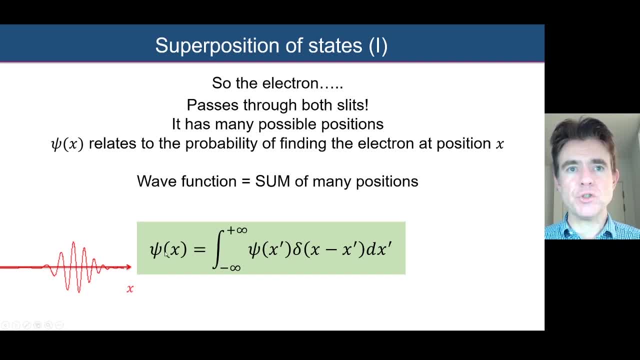 But we're saying we can add together many of them to actually create that single wave form. So I refer you to an earlier video where I've described that in detail. So for now I just want to remind you of the superposition of many positions that describes a wave function. 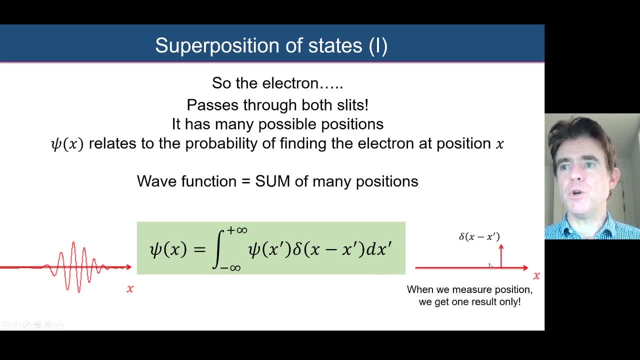 And just a reminder here that when we do this, when we do make a measurement, we only end up sampling from and getting from, just getting just one position from that wave function, And so that's a single delta function at a particular location, for example x prime. 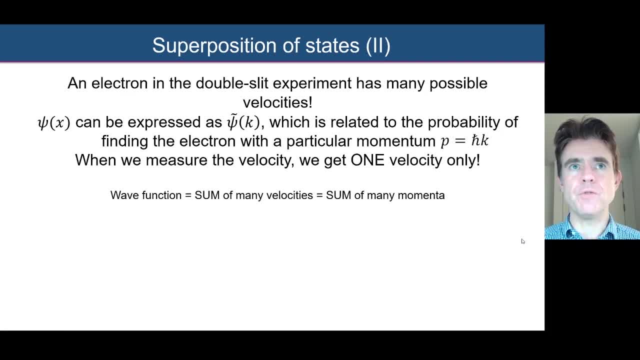 Now, the same can be said from the point of view of measuring the particle velocity. So whereas before we saw that the wave function could be expressed as a summation of position states, it can also be expressed as a summation of momentum states. 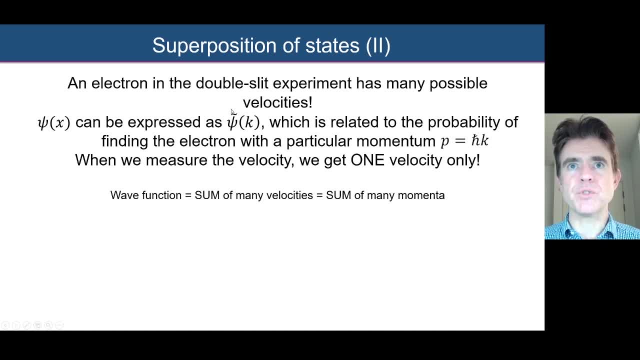 each with a particular amplitude as well, where here I'm using psi with a tilde on the top to denote that this is the amplitude associated with a particular momentum which is related to a particular spatial frequency. k. Remember the relationship: p equals h cross k. 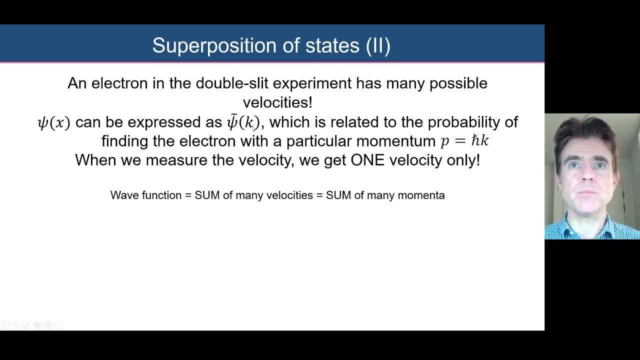 So k and p, spatial frequency and the momentum, are very much related in quantum mechanics, just related by h bar or h cross. Okay, So therefore this relates to the probability, this psi- with a tilde on the top- as a function of spatial frequency k. 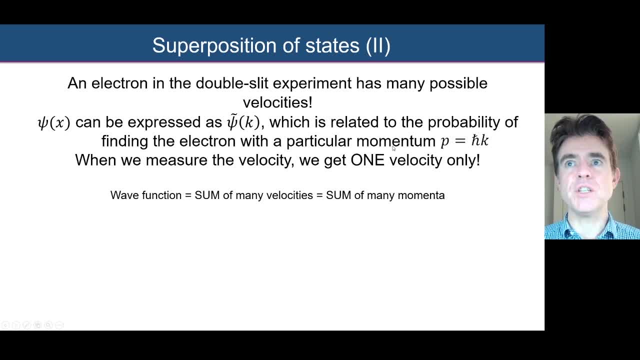 is related to the probability of finding the electron with a particular momentum k, or measuring the electron to have a particular momentum k, or rather I should say spatial frequency, which of course directly infers momentum. Okay, So therefore the wave function now is also a sum of many velocities or a sum of many momenta. 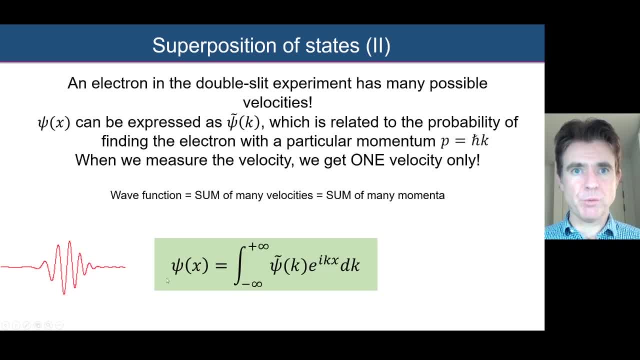 So that would look something like this, where we've got a wave function now and we're saying it's a summation over many momenta. So a fixed momentum just corresponds to one wave function, e to the i, k, x, where k is fixed. 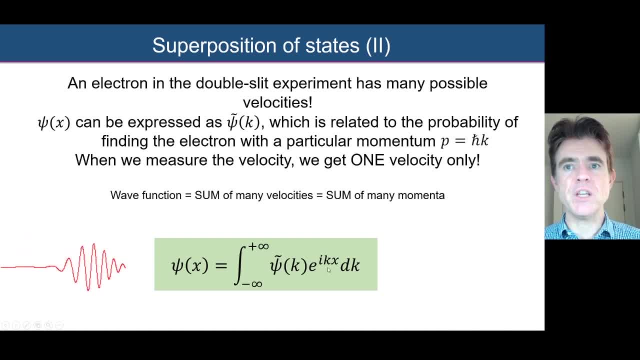 just one value of k by p equals h cross k. one value of k means one value of momentum, And so that corresponds to a cos plus an i sine function. But when we add those together with various amplitudes and sum them all together, 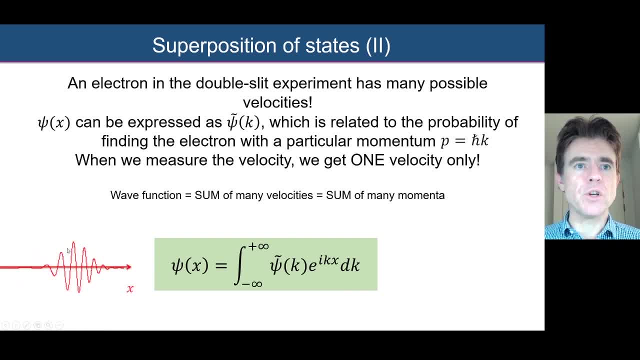 we create a wave function which might look, for example, something like that at a fixed moment in time, And so, notice, we are expressing this just as a function of space spatial coordinate with fixed time here. So it's the time independent wave function that we're looking at here. 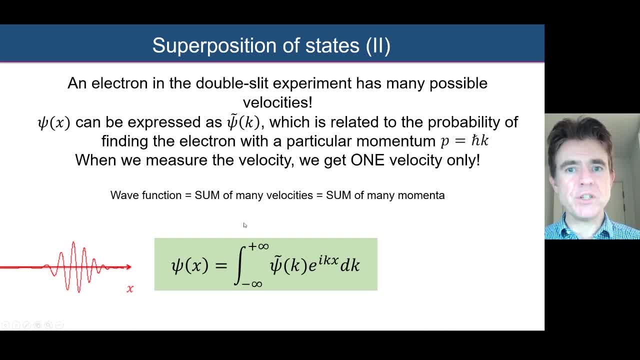 And that's how it might look. Now. if we attempt to measure the momentum, then, a bit like with the position situation again, the wave function will collapse and only correspond to one fixed momentum that we measure. And if we only measure a fixed momentum, 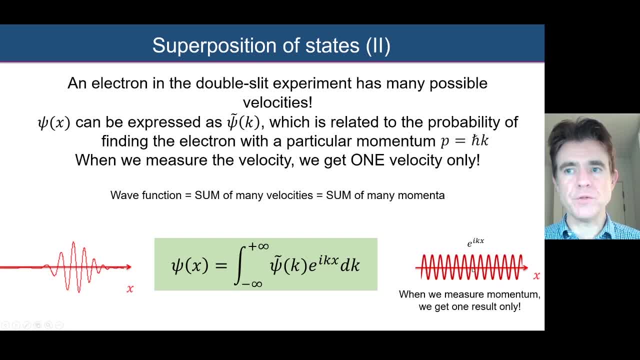 that means that wave function has become now just one of these complex exponentials which corresponds to a fixed value of k, a fixed value of momentum, a fixed value of the velocity. So that is another example of wave function collapse, And the collapse depends on the kind of measurement that we are doing. 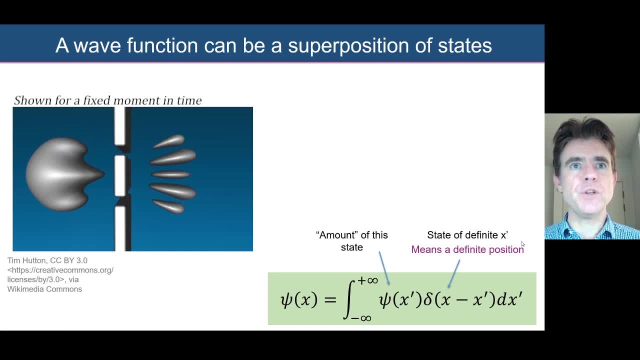 So this is just a summary of that. So here is an example again of that wave function passing through the double slits And this is expressing a probability amplitude as a function of position. We can express that wave function as a superposition of positions. 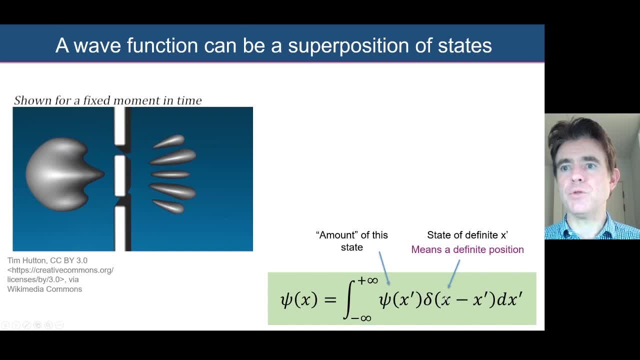 So we've got definite positions here and we've just got amplitudes of each of those possible positions. When we measure it, of course, remember when we measure this on the screen, we just get one dot, one fixed location. 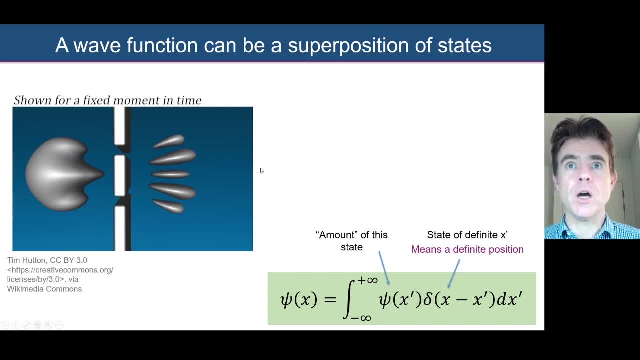 which will correspond to when that wave function reaches the screen. we'll just be sampling one position from it and only having that one piece of information. But alternatively, we could also express it as a summation of momentum states, And so that's what this expression is doing here. 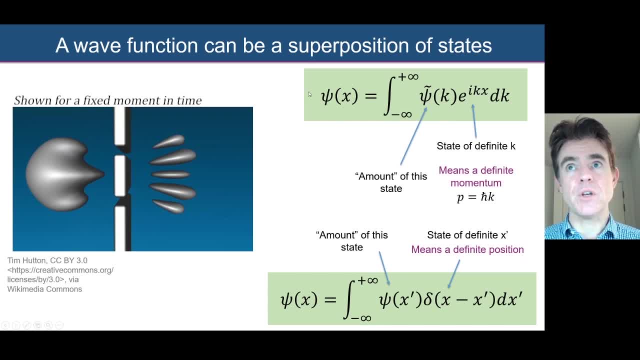 And effectively this is better known as an inverse Fourier transform, where what we're saying is we're expressing a function of a spatial coordinate as a summation of frequencies, A summation of spatial frequencies. So e to the, i, k, x, that's cos plus i sine. 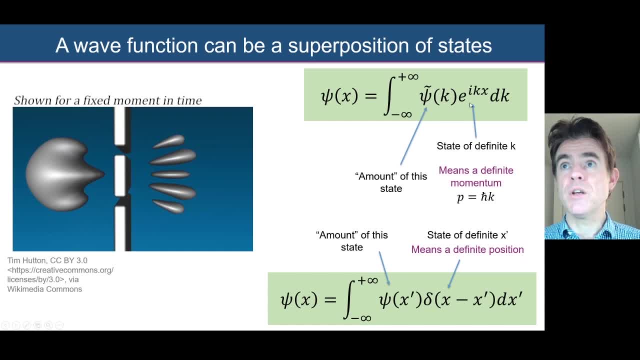 as just mentioned, And then we've got a particular amplitude, a particular coefficient for each one of those complex exponentials. And then we add up all of the possible momentum values for the k running from minus infinity to plus infinity, add them all up with their special amplitudes. 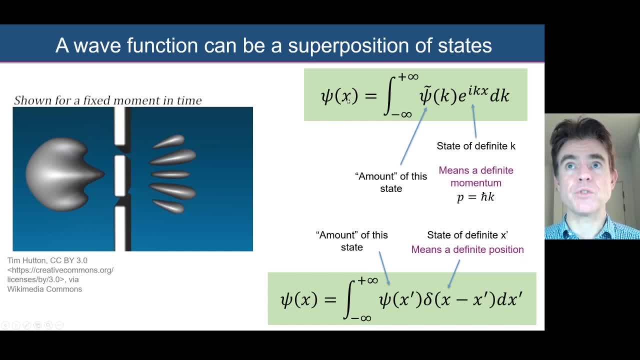 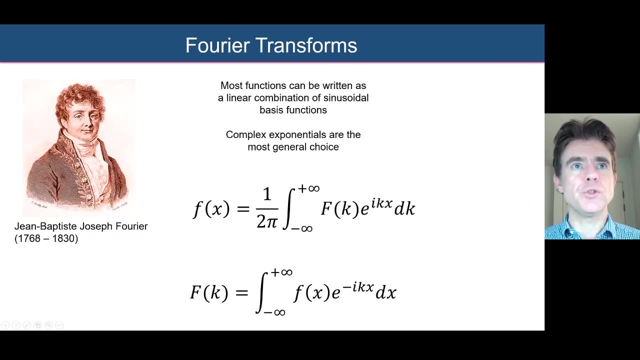 and that will recreate that wave function, psi of x. And so in the next few slides I'm going to demonstrate how this actually works. How does this expression for the inverse Fourier transform actually function? So the Fourier transform. this dates back to Joseph Fourier. 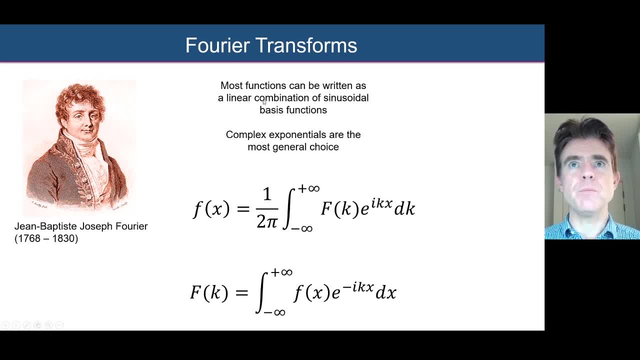 a sketch of him here. And basically the Fourier transform is saying that most functions can be written as a summation, a linear combination of sinusoidal basis functions, And here we'll be focusing on the most general case of complex exponentials, which fit in nicely. 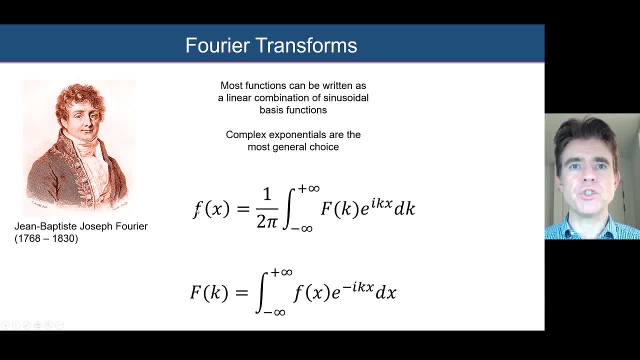 with quantum mechanics. So we're saying, therefore, that a general function f of x is equal to a summation- that's the integral and elongated s- a summation of complex exponentials And each complex exponential. remember that's just a cos and a sine. 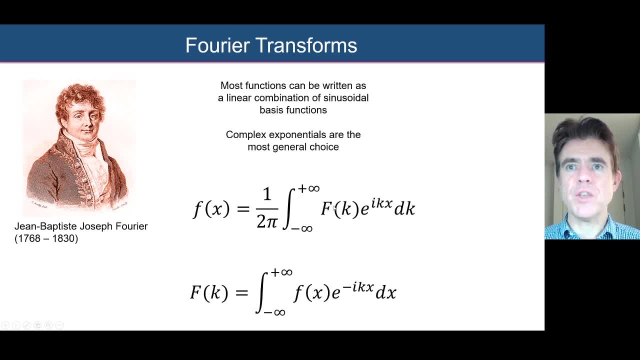 just has a coefficient of capital F, And that coefficient depends on the frequency k. In other words, we get a different amount of each frequency k, And when we add these together in differing amounts, that is what allows us to generate all kinds of general functions f of x. 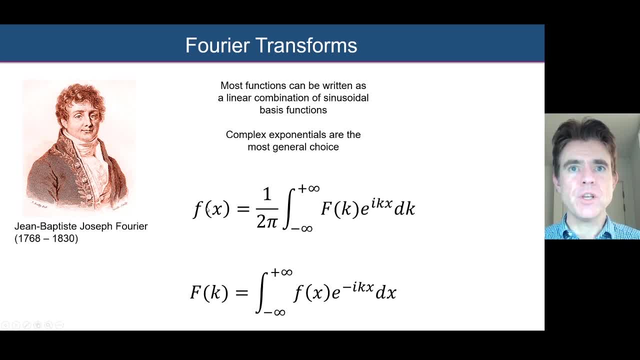 on the left-hand side there, And the key question is: if we want to do this Fourier synthesis, this inverse Fourier transform, how do we go about actually finding the coefficients or the amplitudes for these complex exponentials? Well, the answer to that is this expression at the bottom here: 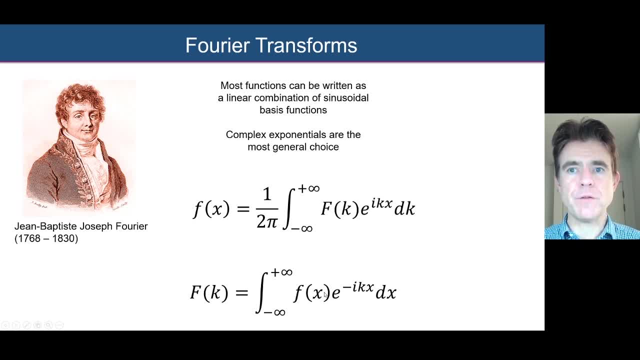 which is the Fourier transform And that says: if you've got a function f of x, if you want to find out how much your frequency k is present in that function, then all you do is multiply the function f of x by e to the minus ikx. 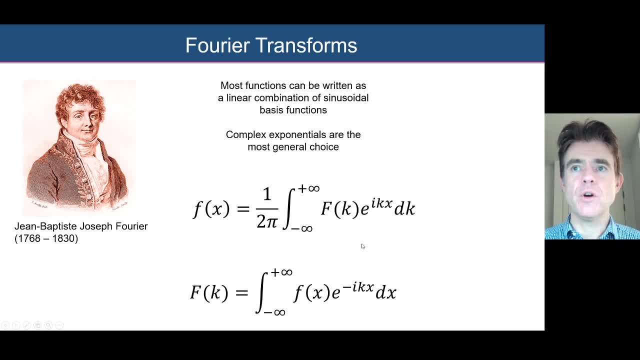 You have to multiply it by the complex conjugate of the complex exponential, And so all you do is just take the negative for the argument of the exponential. So multiply it by e to the minus ikx. The reason for that is we're trying to pick out e to the ikx. 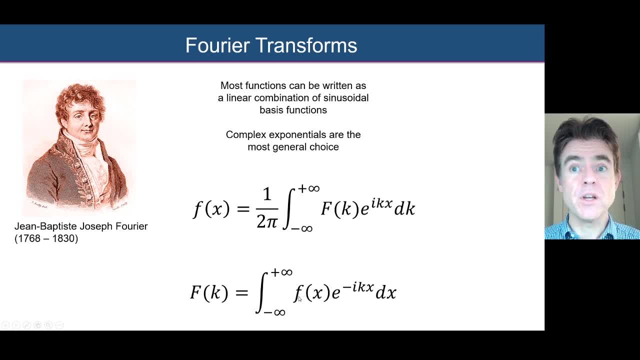 that's present in f of x. If you want to pick that out, then it's going to have to latch on to the case of e to the minus ikx multiplied by e to the plus ikx, which is equal to e to the zero. 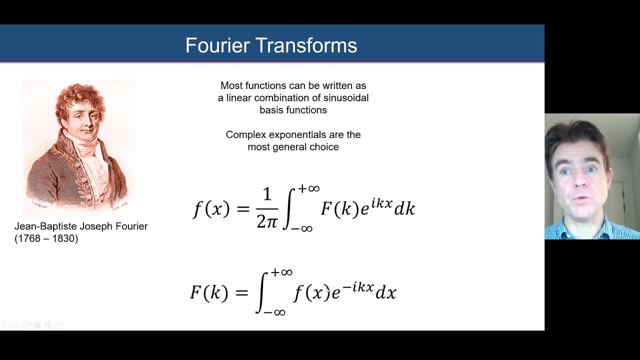 which is equal to one and will give us a finite result, Whereas when this is multiplied by any other complex exponential of a different frequency, it will give a zero result due to orthogonality of these functions. So that's a very rapid overview. 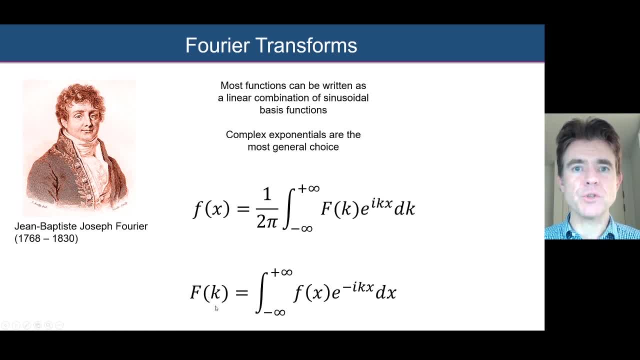 of how the Fourier transform works, And that will give us the amount of each frequency k that is present in f of x. We've got the amount of each frequency k. We can then use that to re-synthesize the original waveform, just by saying. 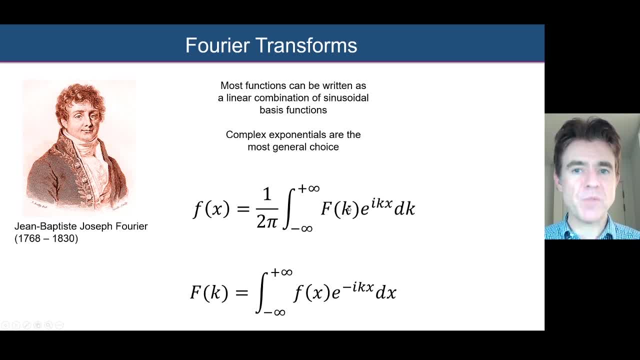 well, we've got the amount f of frequency k. Let's use that as the coefficient for frequency k, which is the complex exponential. Sum them all up and that gives you the function again. So let's take a look at these maths formulae. 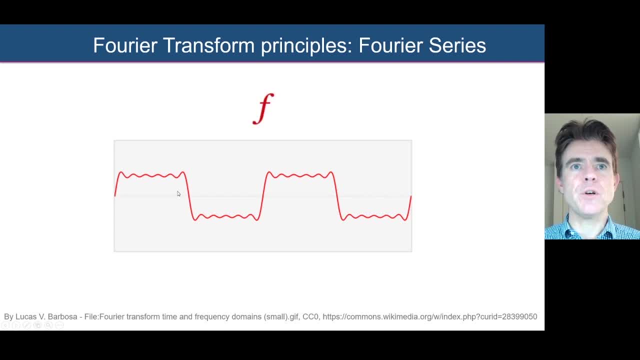 by practical examples. So here we have basically a square waveform. This is more like a Fourier series, And we're saying, we can add together multiple sine wave functions or indeed cosine functions with different coefficients. Here is a, n and b? n. 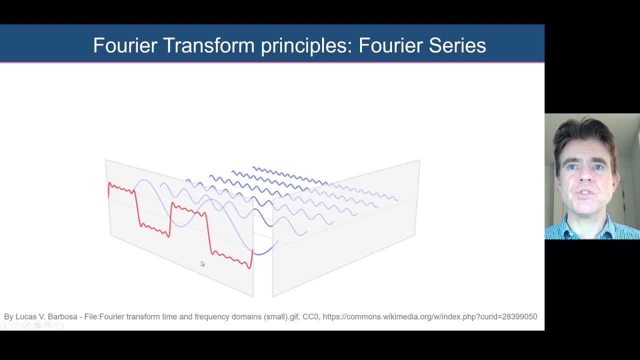 We're adding them together to create that red waveform. So now we're going to see the decomposition of all these. look like sine functions being added together with different amplitudes shown on that right-hand side there When you add them together with those amplitudes. 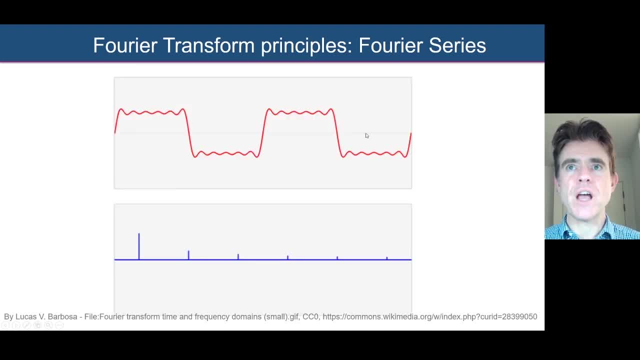 you re-compose, you synthesize that red function. So this told us how much of each frequency you can imagine. the frequency axis along there tells us how much of each frequency to add together to fabricate, to actually reconstruct or synthesize that red waveform. 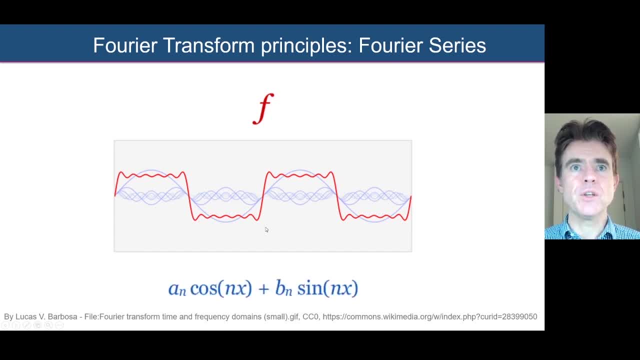 So there it is again. There are the blue constituent components to that red waveform, And we'll just see it one more time to see the breakdown. That red waveform is equal to a summation of all of those sinusoidal functions. So in quantum mechanics, 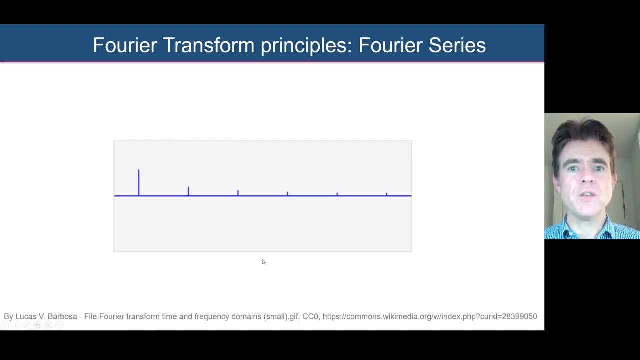 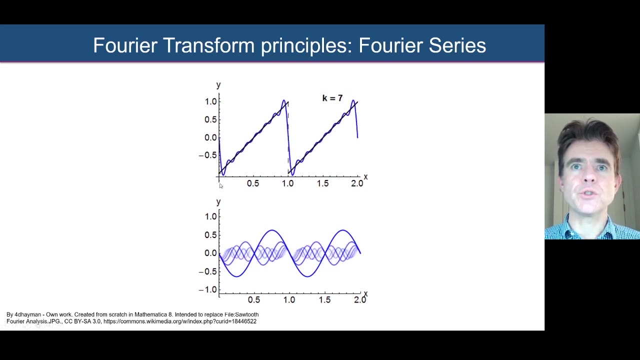 that's like saying if our wave function looked like that red function, then it would be composed of many momentum states given by each of those sinusoidal functions. Okay, so here is the Fourier series, again showing that this sawtooth function, this kind of linear function,